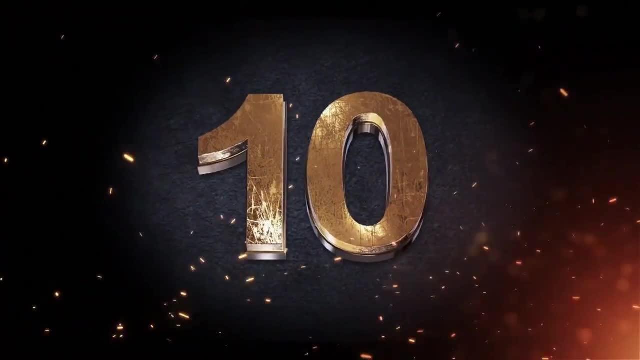 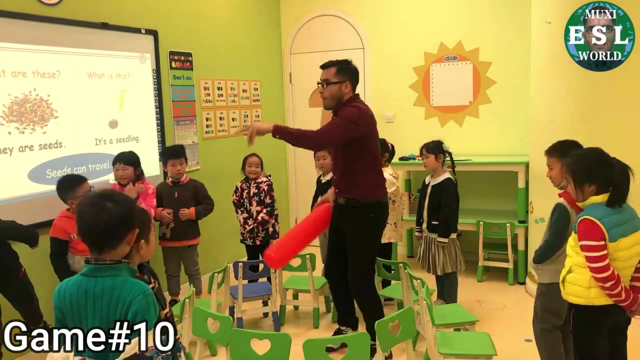 What we said Eight minutes. When you hear Jay ring the bell, you're going to find a chair and sit down If you couldn't find a chair. if you find a chair, then Mushi spoiled himself and then hit you like that. 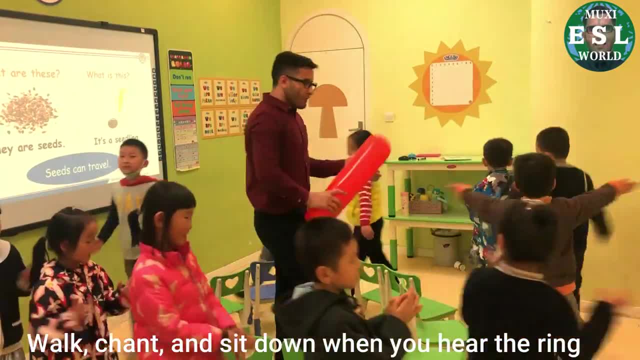 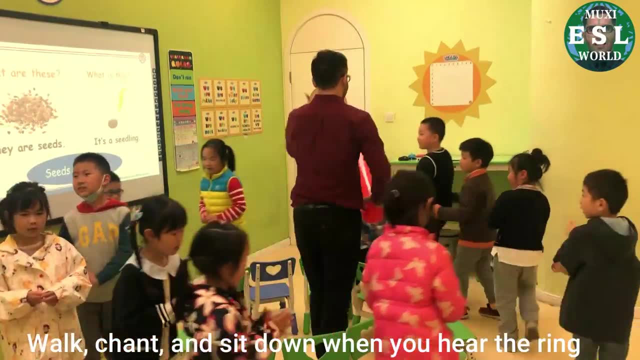 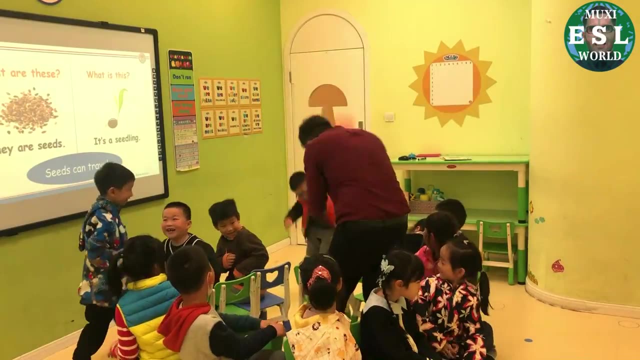 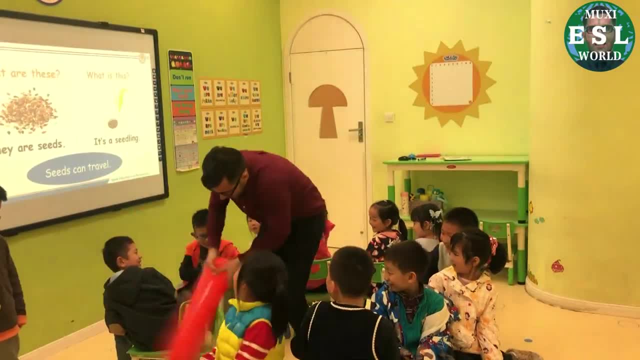 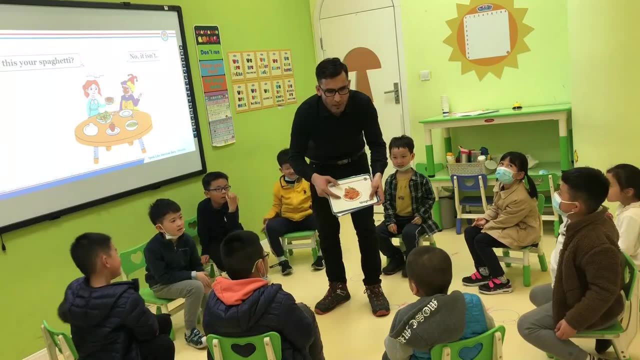 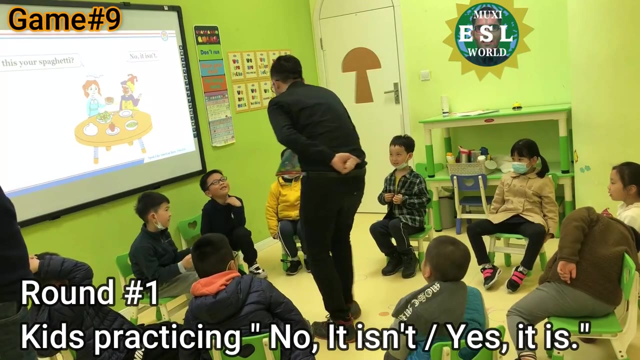 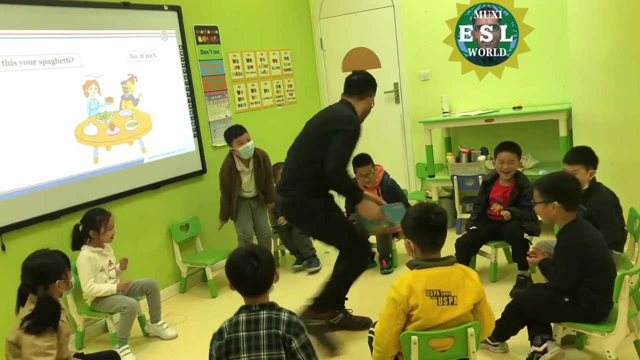 Stop, stop, stop. Start with spaghetti, ok. Is this your pizza? No, it isn't. Is this your ice cream? No, it isn't. Is this your meat? No, it isn't. Is this your spaghetti? 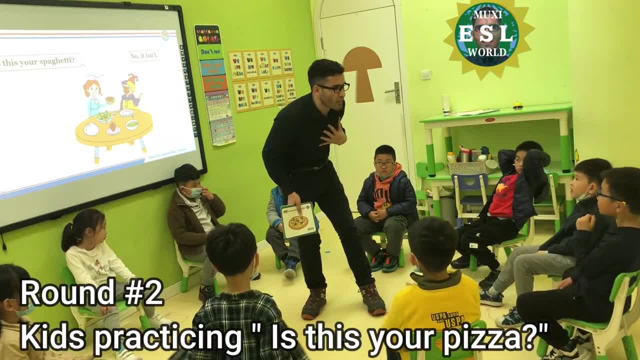 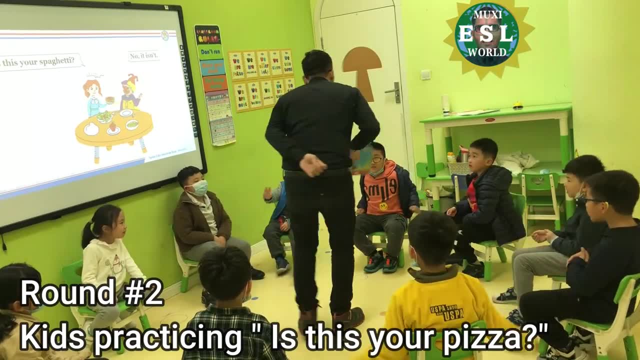 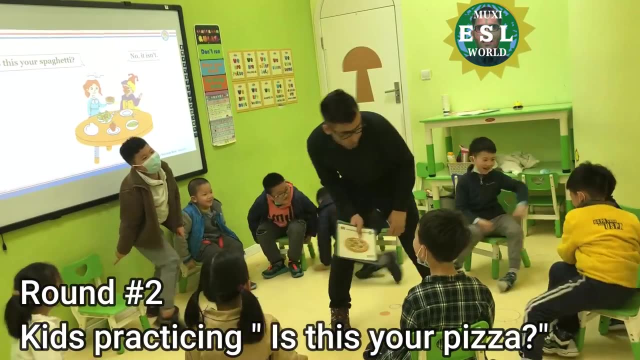 Yes. When I say yes it is, you gotta change your chairs. Is this your pizza? No, it isn't. Is this your pizza? No, it isn't. Is this your pizza? No, it isn't. Yes, it is. 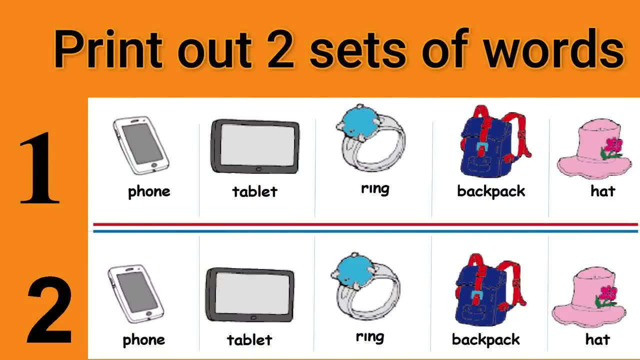 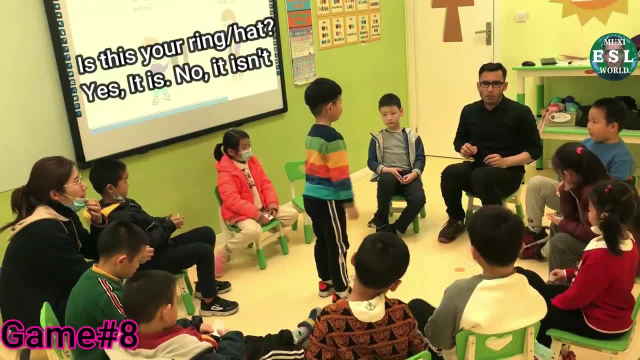 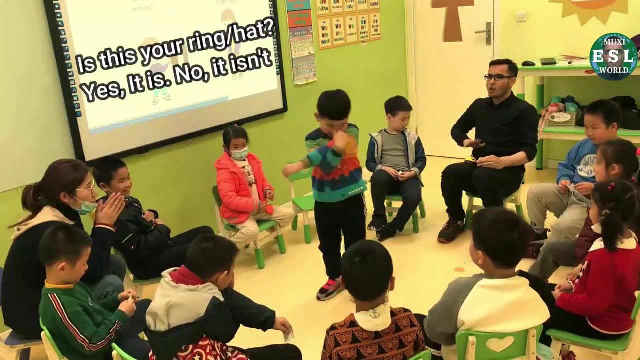 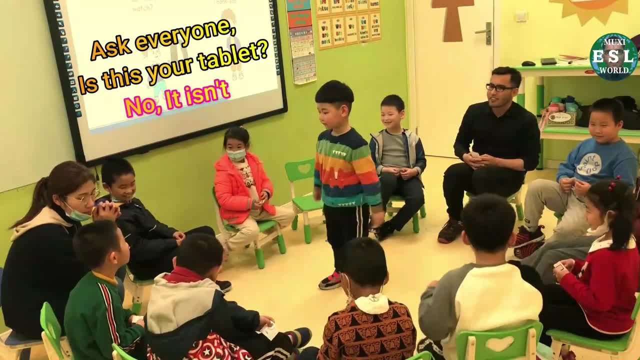 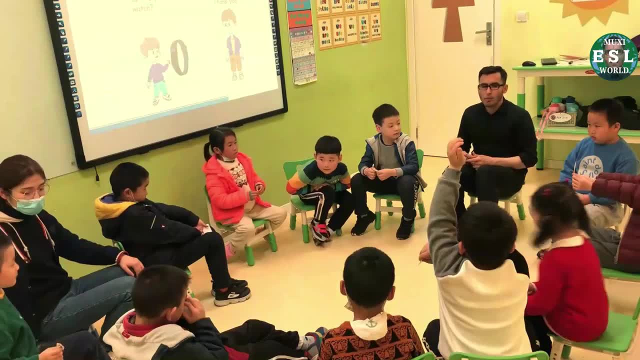 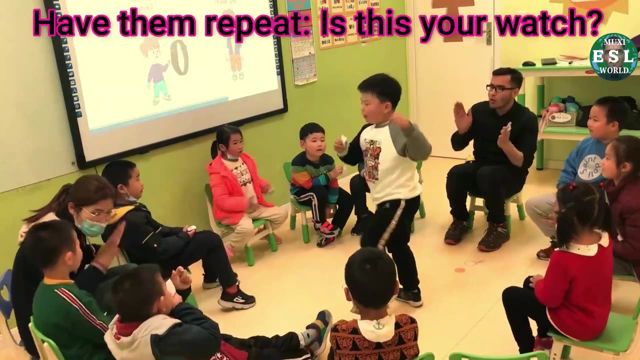 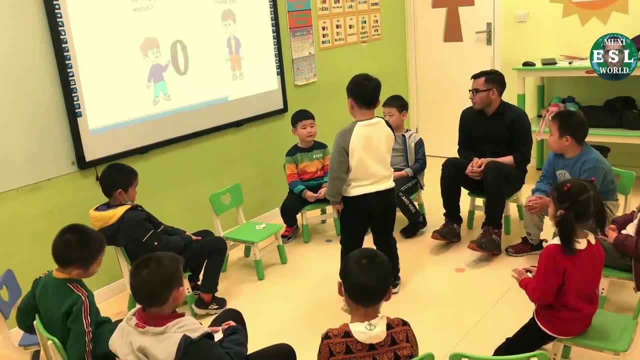 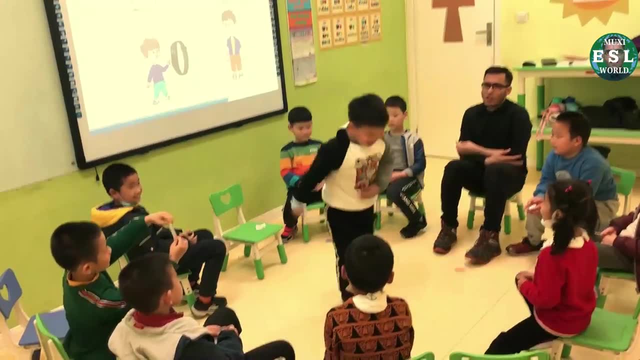 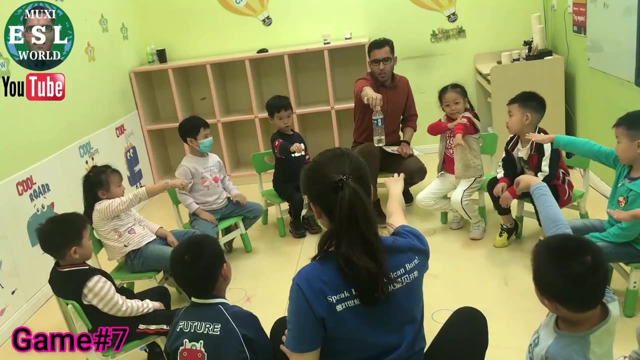 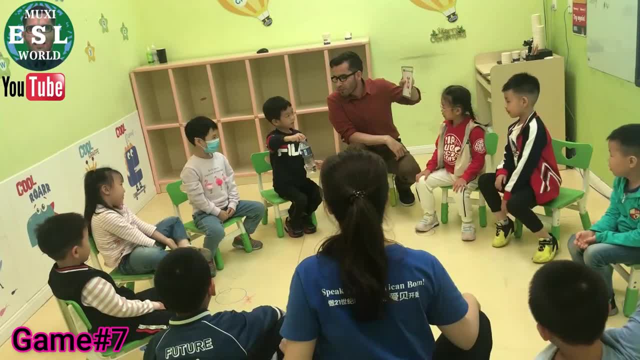 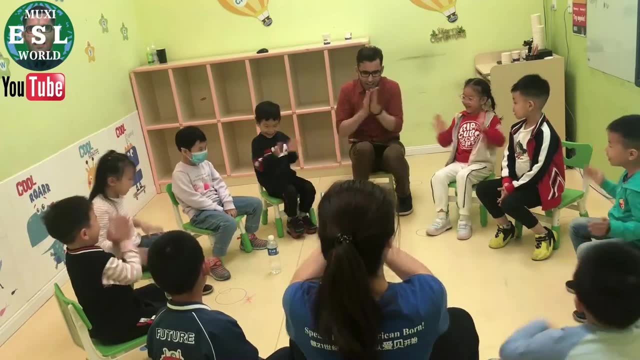 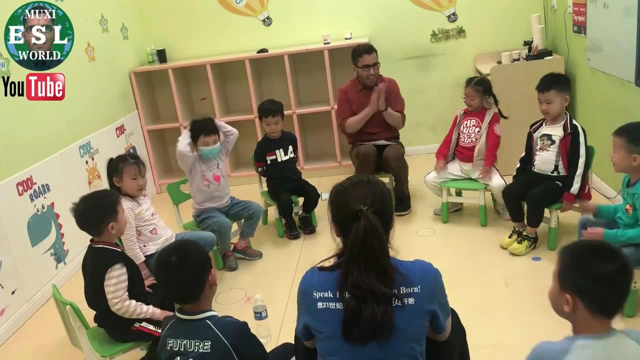 We got it. What number is it? It's number 15!. Yay, What number is it? It's number 15! Yay, What number is it? It's number 15! Yay, Your turn Jackson. 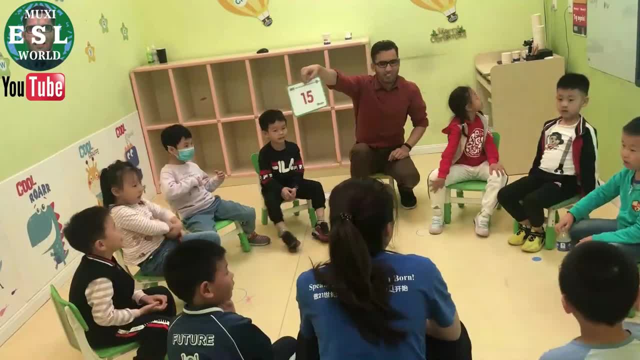 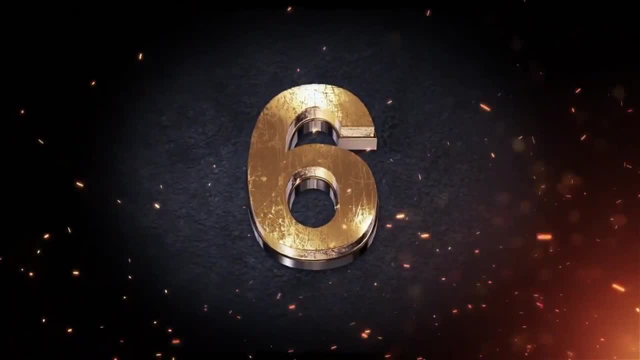 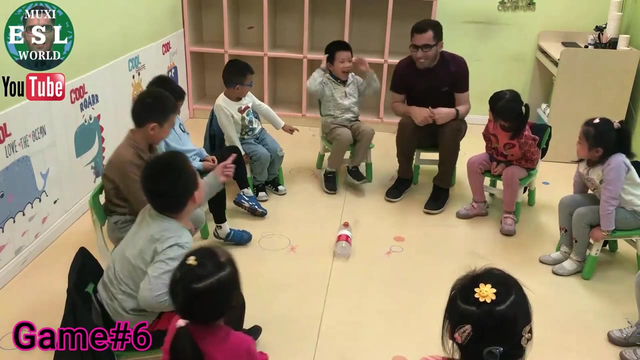 Let's everybody ask: We are happy, we are happy students, We are respectful And we are kind, And we are kind, Let's play another game. Let's play another game. we say: spin the bottle Ready, Ready Now. J-A-P-P. Amazing, good job Patrick. 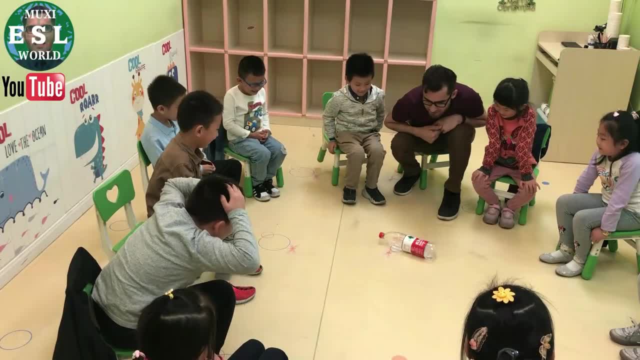 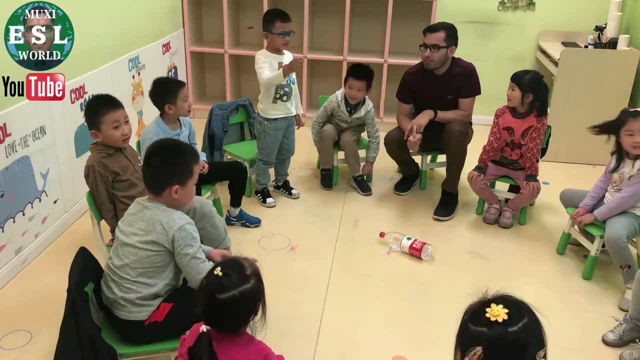 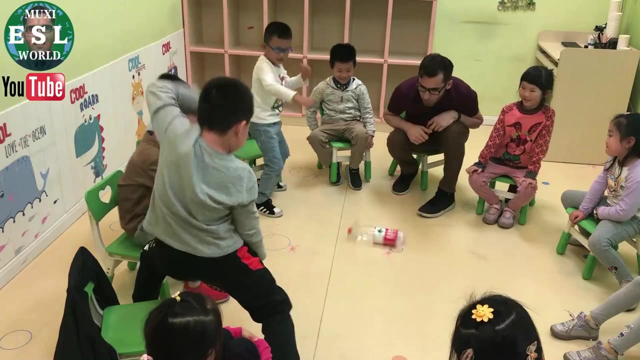 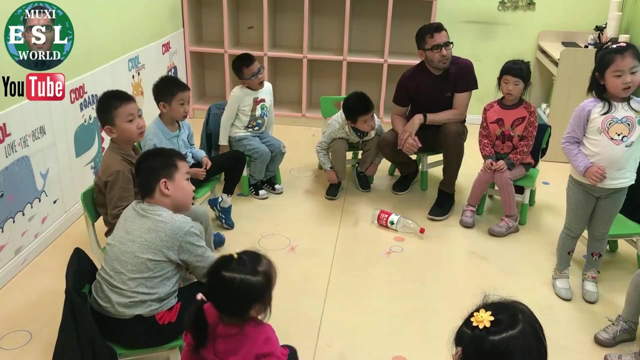 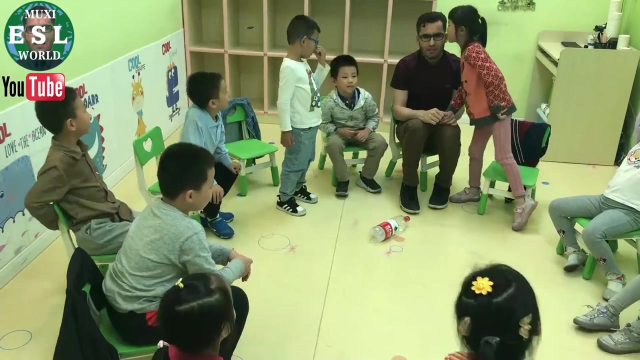 Ready, Wow, Wow. B-O-X, B-O-X Box Box. Good job. thank you, Dread No Mumu H-O-T Heart. Brilliant job, Mumu. We explore, we create, We explore, we create, We explore, we create. 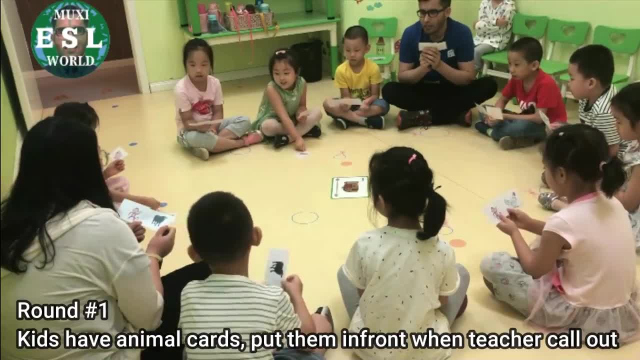 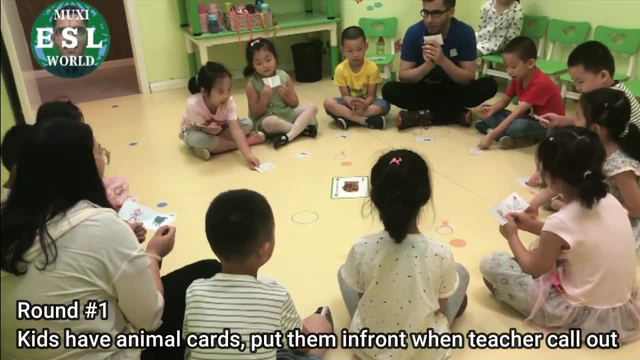 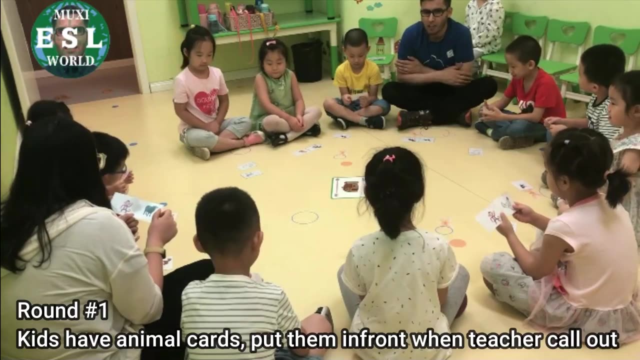 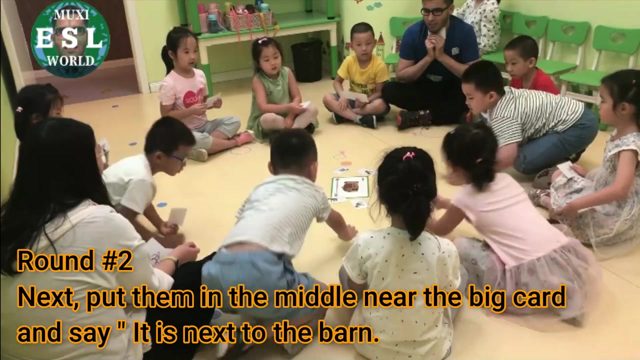 Where is the cat? Here it is. Where is the cow? Here it is. Where is the rabbit? Here it is. Where is the lamb? Here it is. Where is the duck? Here it is. Where is the chicken? It is next to the barn. 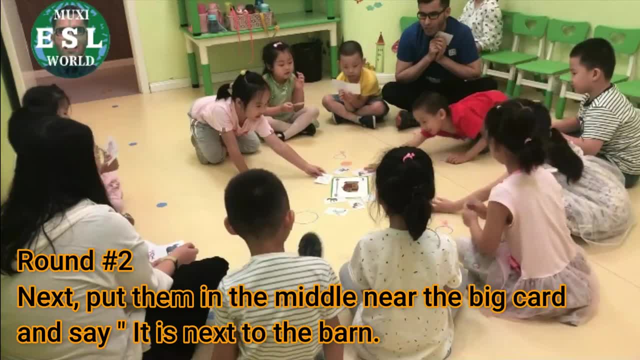 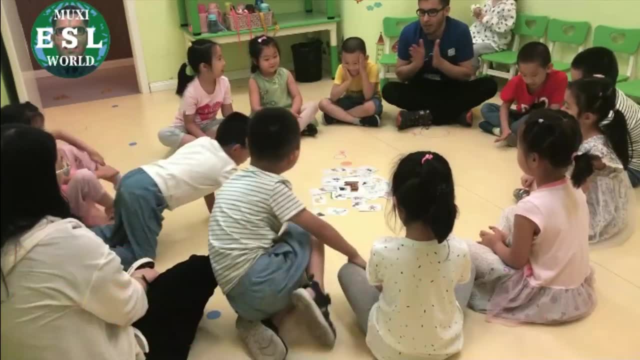 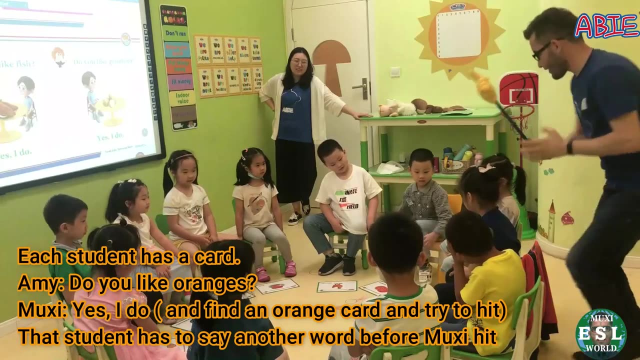 Where is the rabbit? It is next to the barn. Where is the sheep? It is next to the barn. Where is the sheep? Where is the sheep? Do you like oranges, Oranges? Yes, I do. Do you like chicken? Yes, I do. 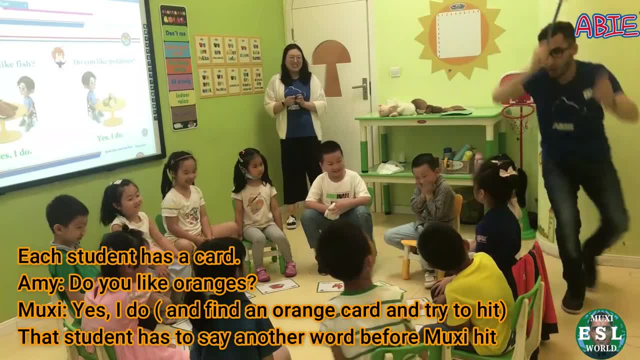 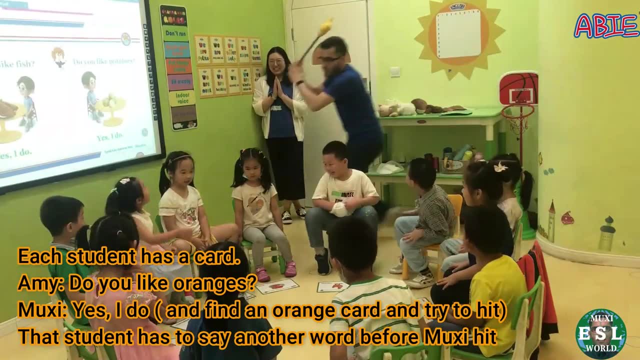 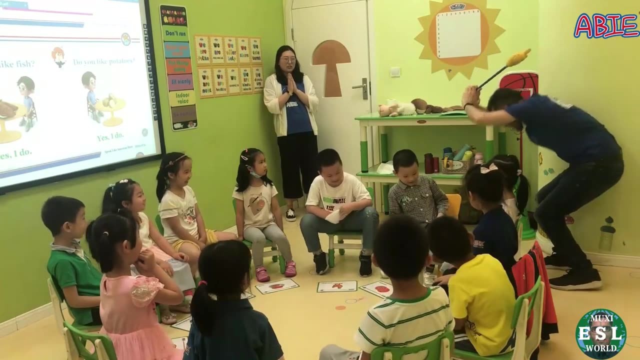 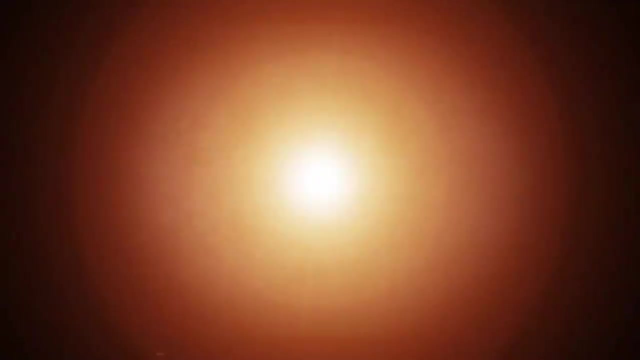 Do you like milk? Milk, Yes, I do. Do you like fish? Yes, I do. Do you like milk? Yes, I do. DO YOU LIKE ORANGE? Yes, I do. Do you like it? Do you like it? Now? Mushi says I. 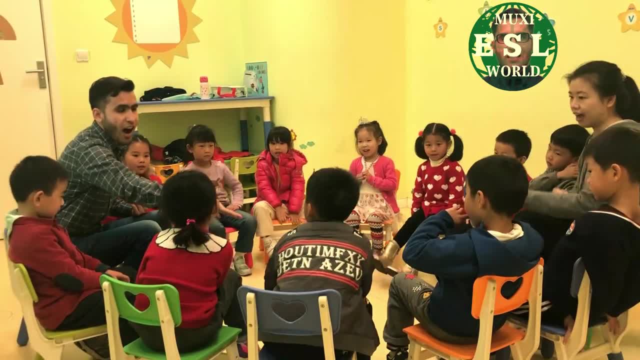 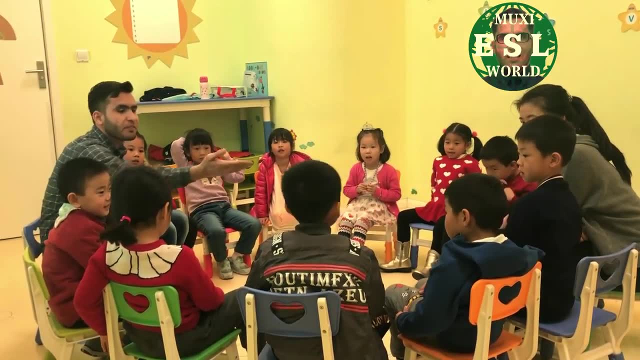 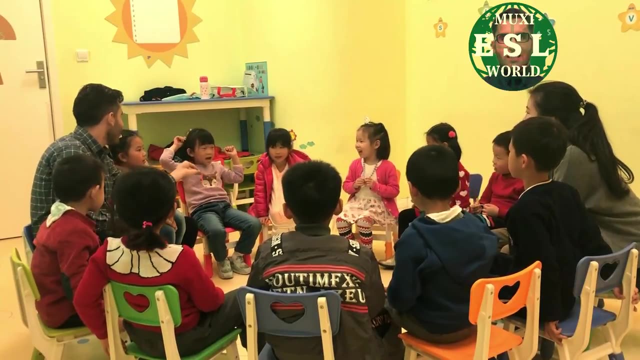 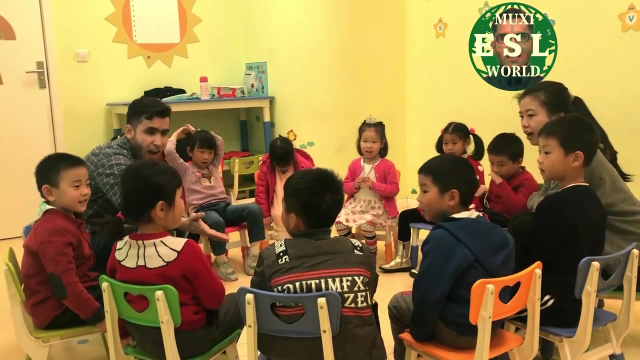 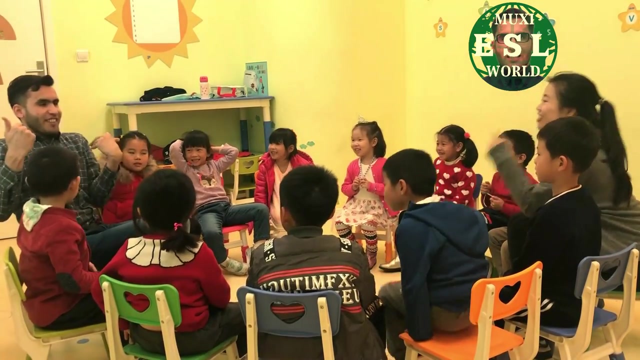 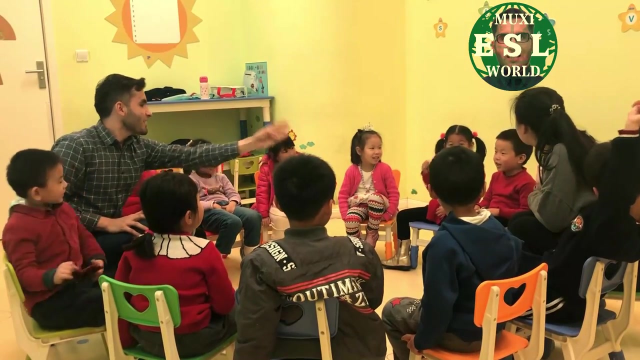 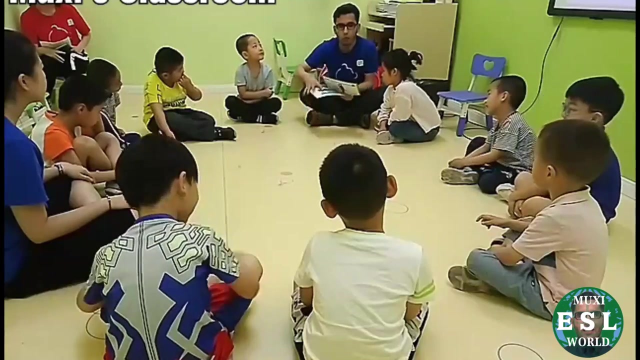 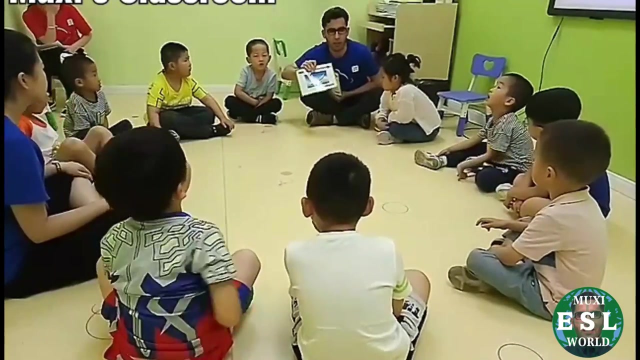 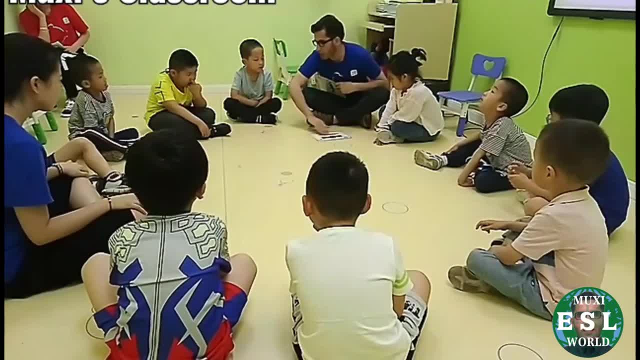 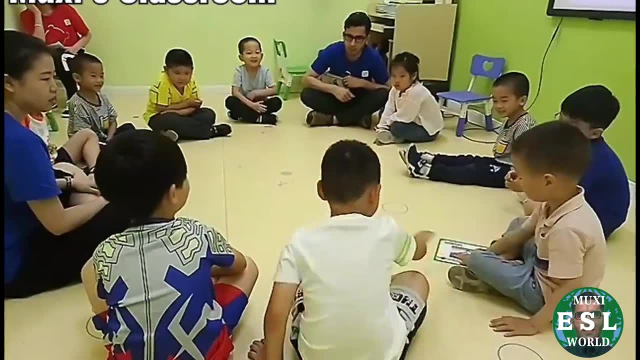 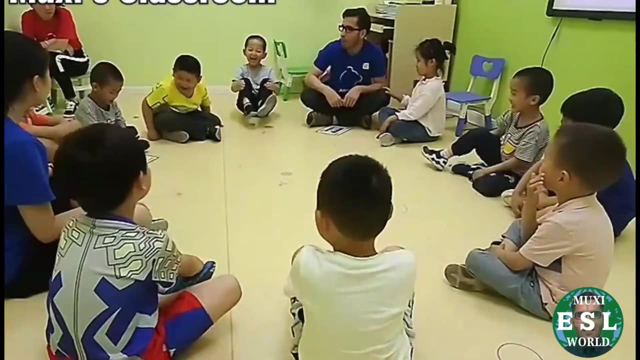 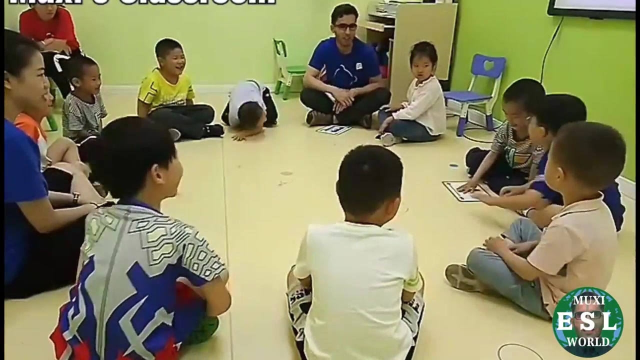 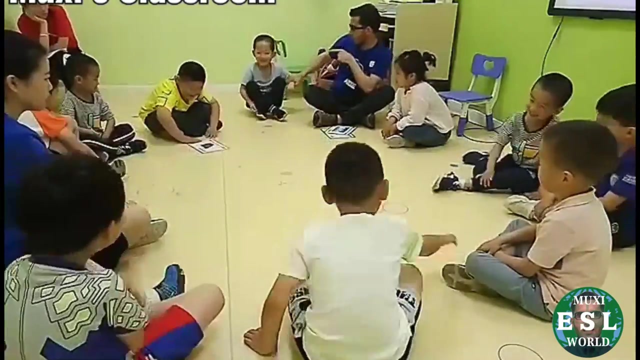 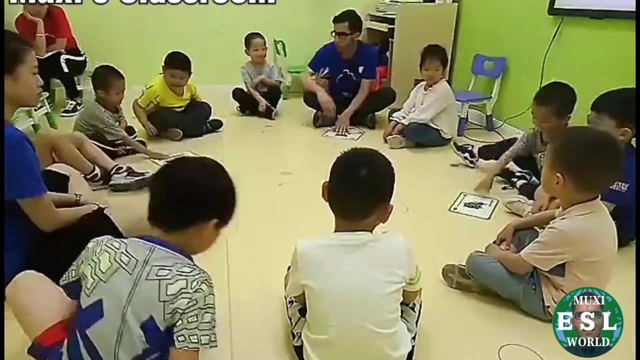 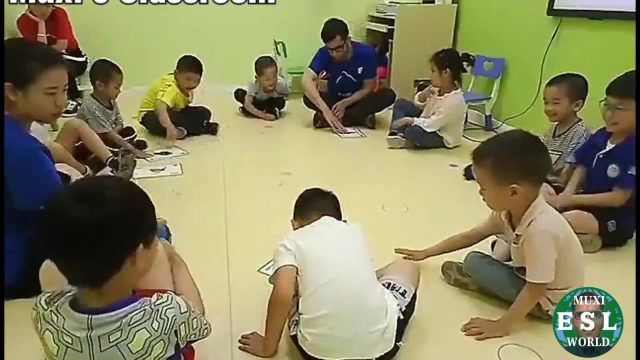 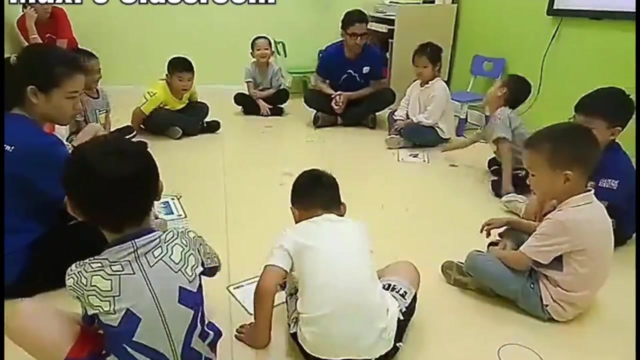 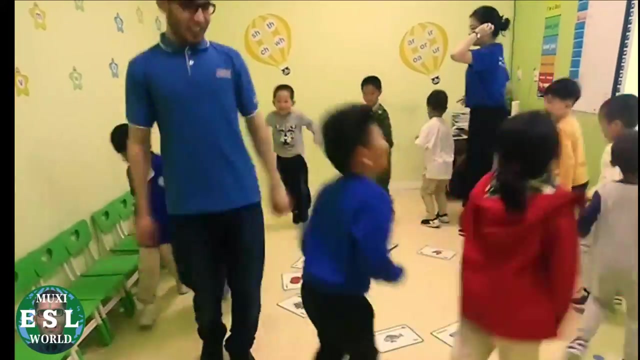 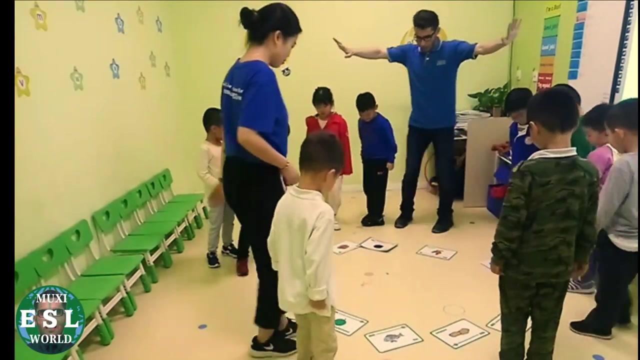 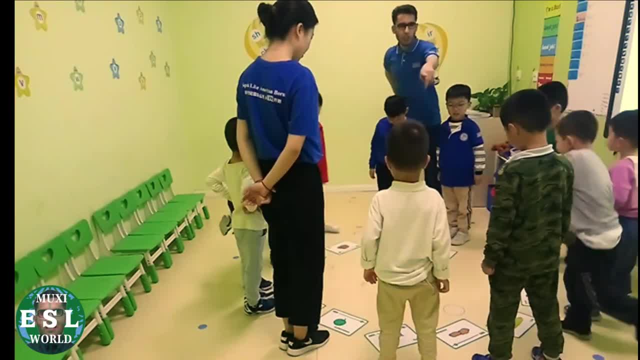 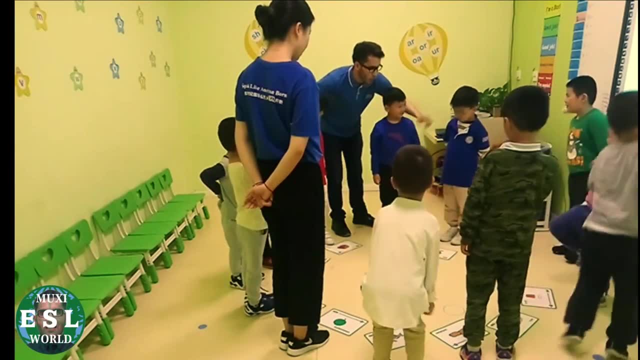 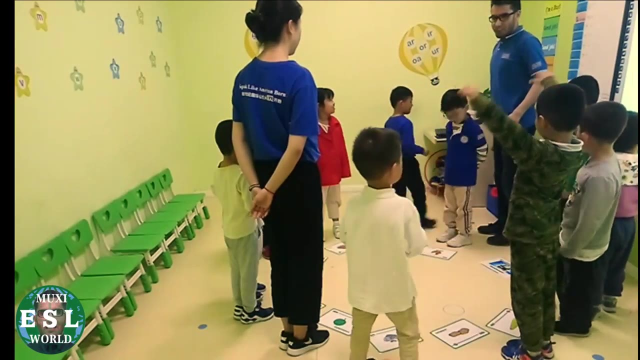 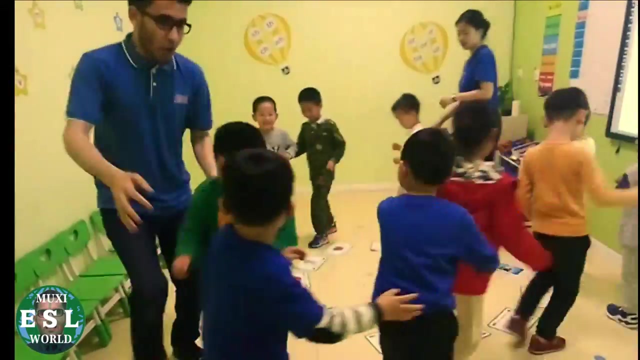 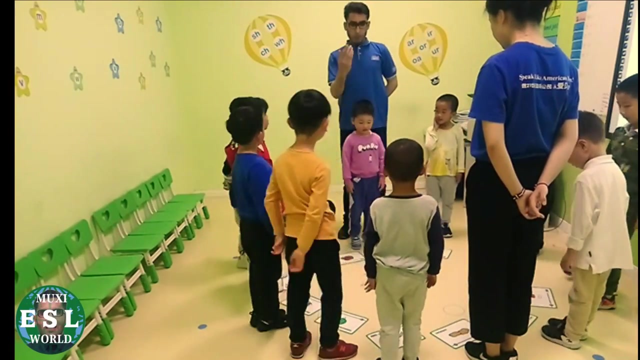 Richard, what do you like to eat? I like fish. You like fish, George, what do We are happy, we are happy. we are happy students. We are respectful and we are kind. We value our friends and we value ourselves. We think, we ask, we think, we ask, we think and we ask, We explore, we create, we explore, we create, we explore, we create. Thank you.